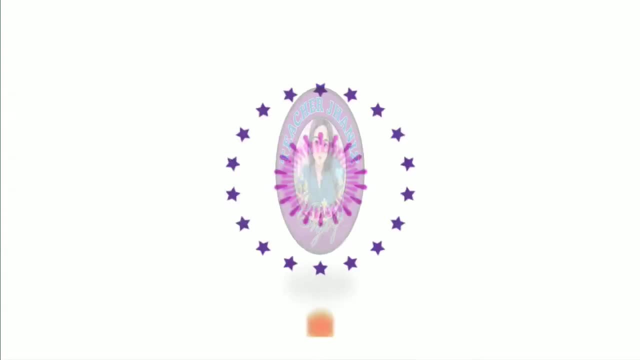 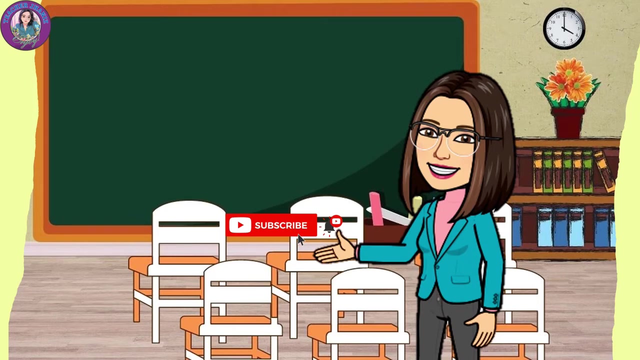 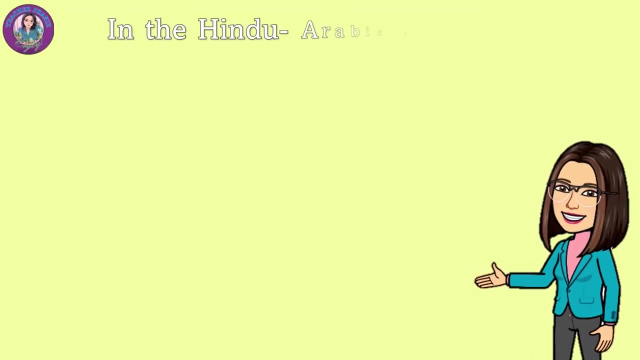 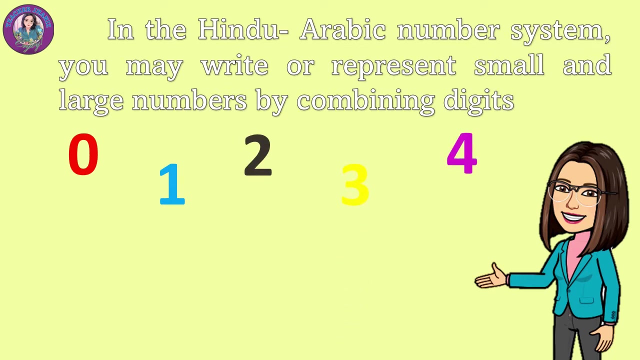 Good day. Welcome to our math class. For today's lesson we will understand whole numbers In the Hindu-Arabic number system. you may write or represent small and large numbers by combining digits 0,, 1,, 2,, 3,, 4,, 5,, 6,, 7,, 8, and 9.. 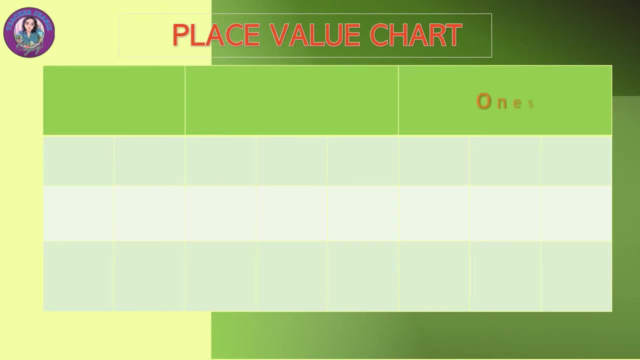 Look at this place value chart. We have 1's Under that, we have 1's place, 10's place, 100's place. Next, we have 1000's Under that, we have 1000's, 10,000's, 100,000's. 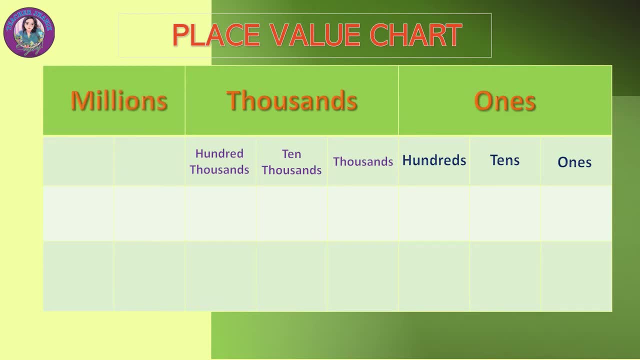 Next is the millions. Under that we have millions. We will find 1's in terms of total number of months. This can be written as none, 100,000, and 10,000,000.. 1's has the value of 1.. 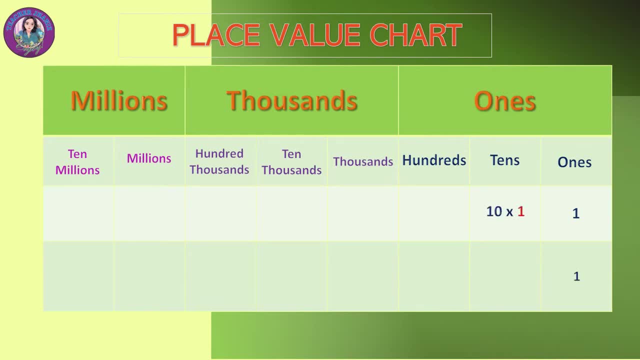 One is 10 times 1.. The number of months is number 10.. H Level is 10.. The 10 times 1 is worth 10.. An nav vibe-�� value 1's has the value of 1.. 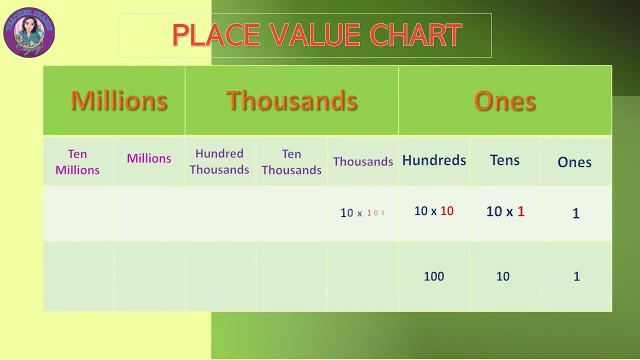 And 10 times 1 is 10.. It's value is 10.. 10 times 10 in the 100's place, its value is 100.. In 1000's we have 10 times 100, In ten thousands we have 10 times 1,000.. Its value is 10,000.. 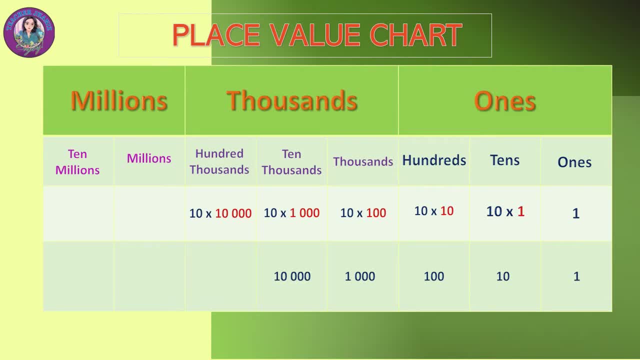 In hundred thousand, we have 10 times 10,000.. Its value is 100,000.. In millions, we have 10 times 100,000. Its value is 1 million. In ten millions, we have 10 times 1,000,000.. Its value is 10,000,000. 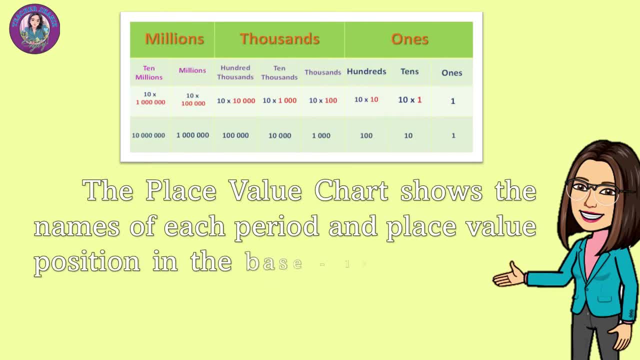 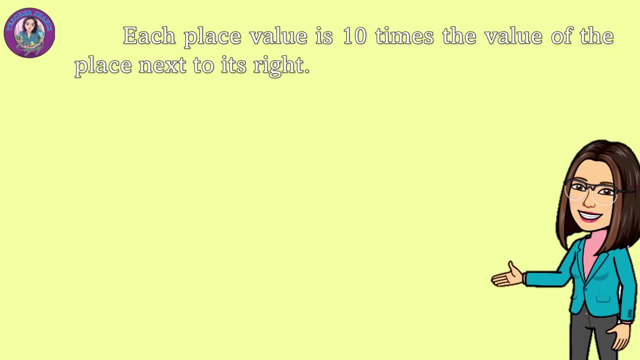 The place value chart shows the names of each period and the place value position in the base-10 numeration system. The place value chart shows the names of each period and the place value position in the base-10 numeration system. Each place value is 10 times the value of the place next to its right. 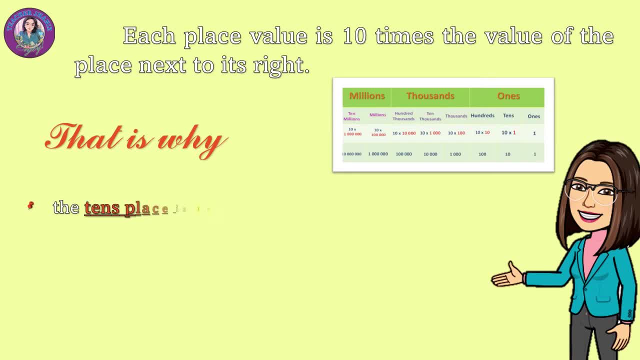 That is why the tens place is 10 times the value of the ones place. It's like 1 times 10 is 10.. The hundreds place is 10 times the value of the ones place. The tens place is 10 times the value of the tens place. 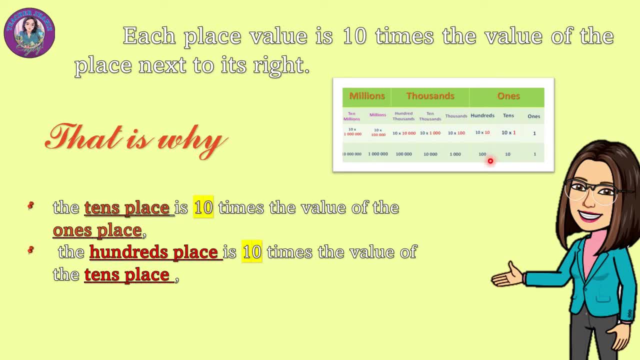 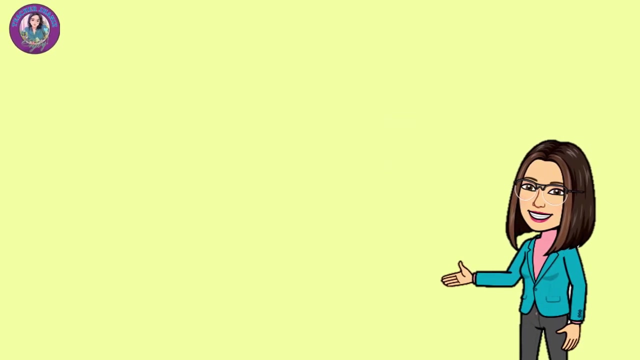 That is, 10 times 10 equals 100.. The thousands place is 10 times the value of the hundreds place. That is, 10 times 100 is 1,000, and so on. For better understanding, let's have this example: 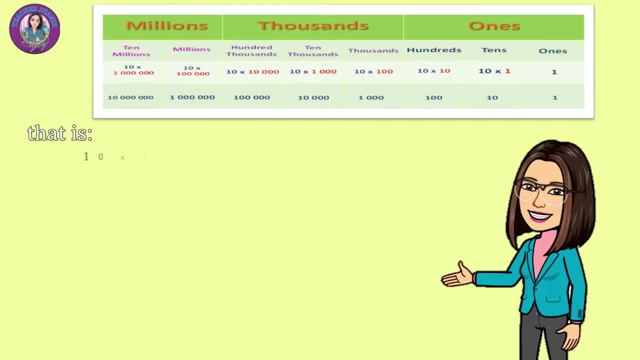 For better understanding, let's have this example: 10 times 1 is 10.. 10 times 10 is 100.. 10 times 100 is 1,000.. 10 times 1,000 is 10,000.. 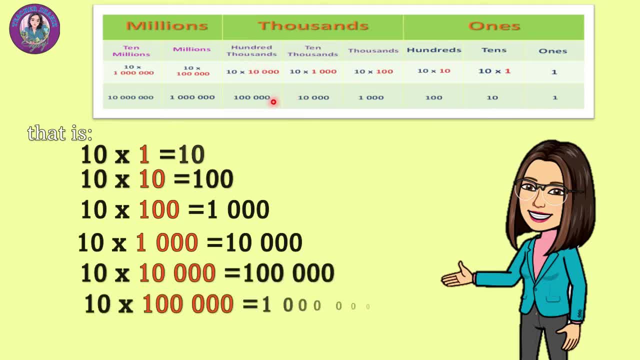 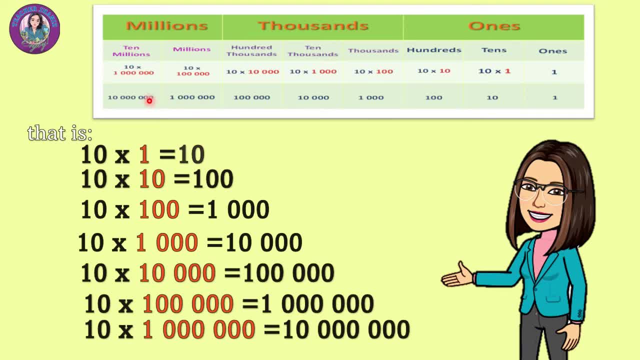 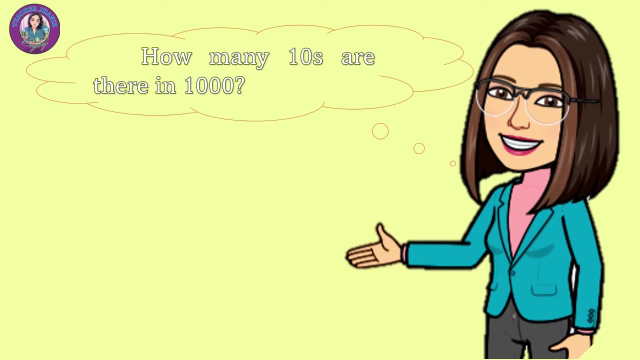 10 times 100,000 is 100,000. This shows that each place value is 10 times the value of the place next to its right. how many tens are there in 1000?? That's right. What is 100 sets of ten? Very good. 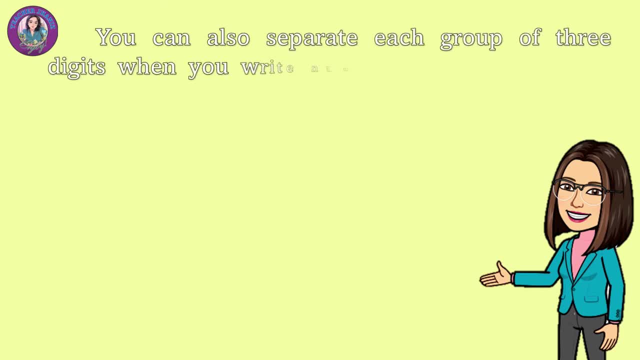 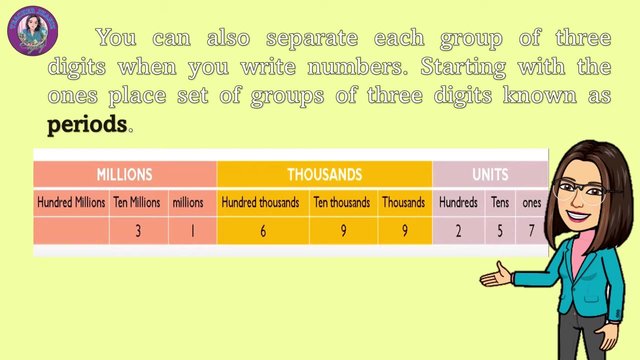 You can also separate each group of three digits when you write numbers starting with a once-placed set of groups of the three digits, known as periods. Look at this chart. In the units period we have the ones, tens and hundreds. 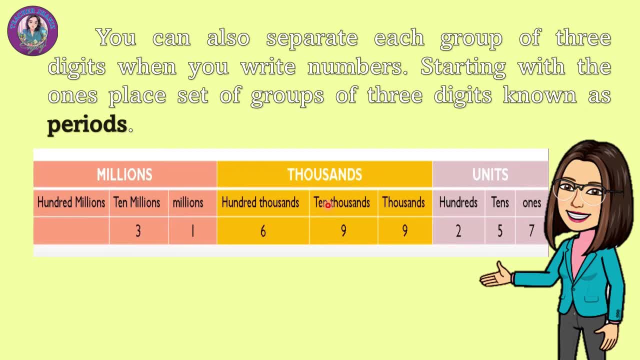 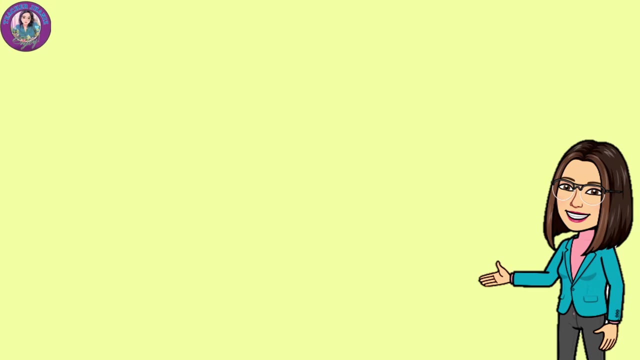 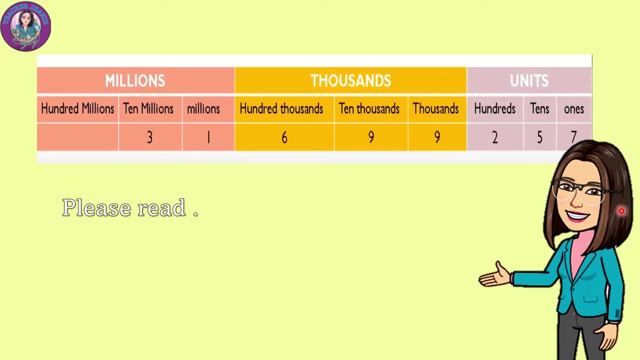 In the thousands period, we have thousands, ten thousands and hundred thousands. In the millions period, we have millions, ten millions and hundred millions. OK, Class, please read using this place value chart: Very good, So we have thirty one million six hundred ninety nine thousand two hundred seventy three. 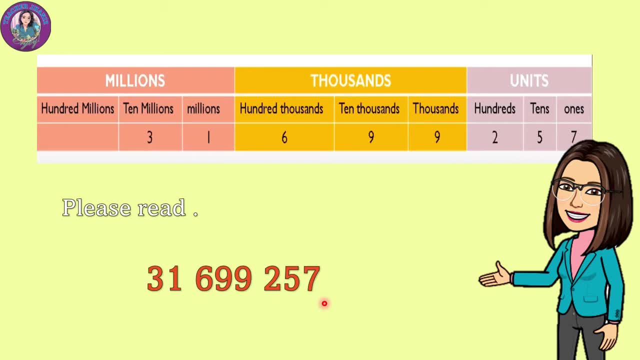 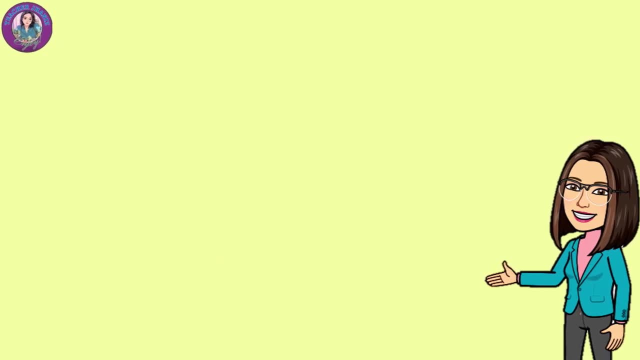 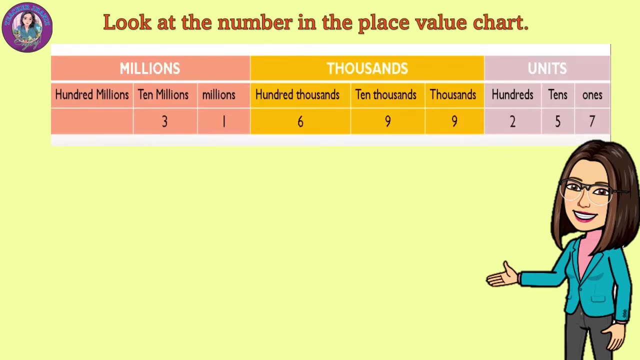 Very good: 31,699,280.. 31,699,280.. hundred fifty seven. look at the number in the place value chart and the ones place you have seven. in the tens place you have five. in the hundreds place you have two. in the thousands place we have nine, ten thousands, nine in hundred. 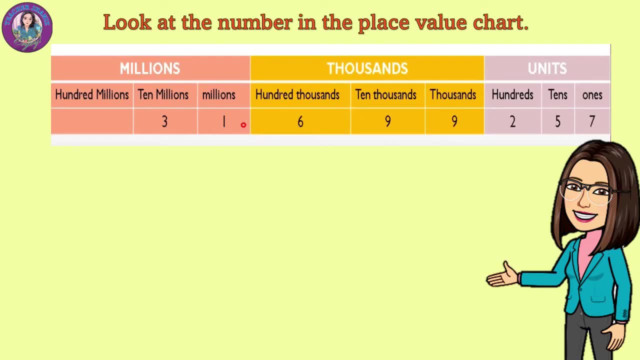 thousands you have six. in millions we have one and in ten millions we have three. the first period is two hundred fifty seven ones. it represents two hundreds, five tens and seven ones. in the second period you have six hundred ninety nine thousands. each represents six hundred thousands, nine ten thousands and 9,000. and the third period we have 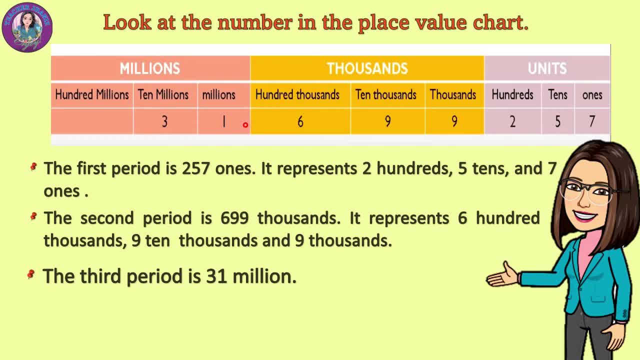 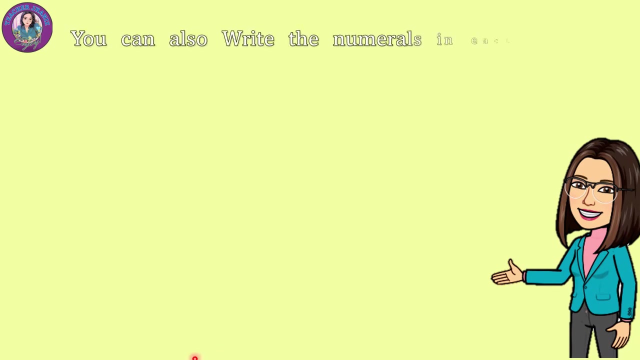 31 million. now what does three and one represents? that's right. three represents 30 million and 1 represents 1 million. you can also write the numerals in each period in expanded form. for example, look at the number in the place value chart. now, if you have 48 and the ones period, its expanded form is zero times 100 plus 4 times. 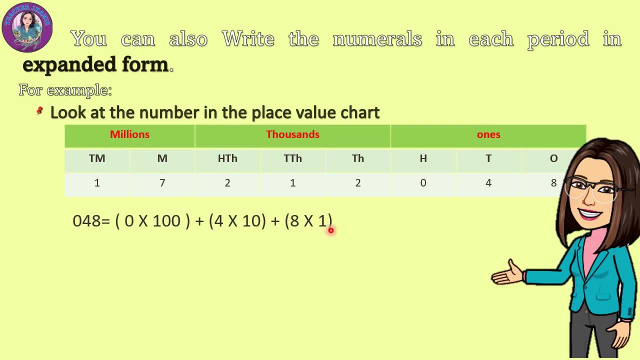 10 plus 8 times one. next, if you have 212 in the thousands period, it's 212 in the thousands period. it's expanded form is 2 times 100,000 plus 1 times 10,000 plus 2 times 1,000. next is: 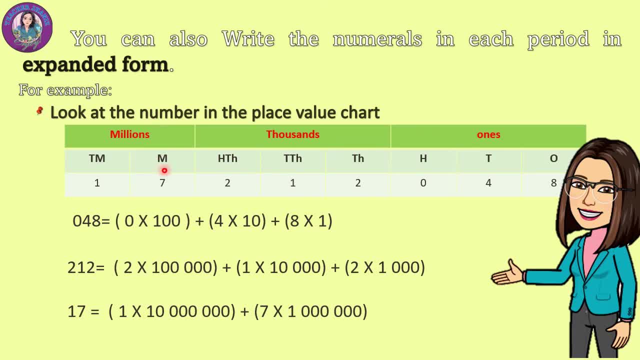 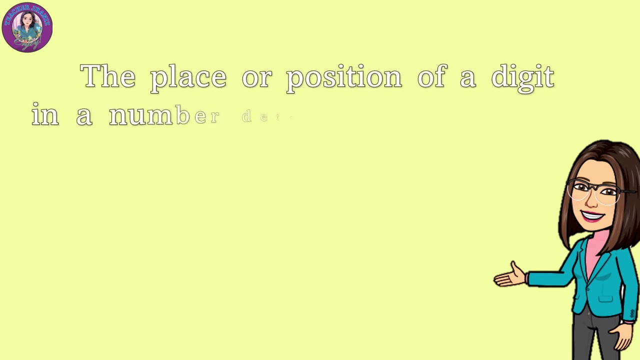 17 in the millions period. so it's expanded form is 1 times 10 million plus 7 times 1 million. now this class that in writing the expanded form. we multiply the digit to its place value. all right, the place or position of a digit in a number. 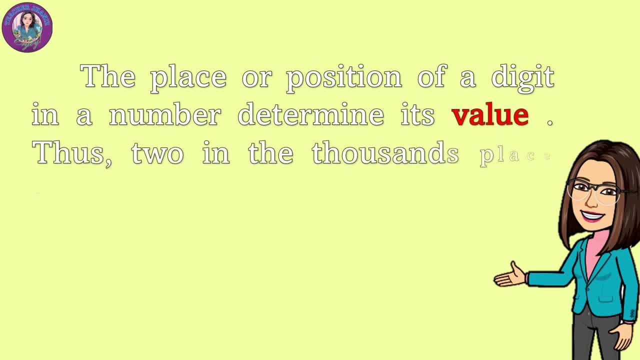 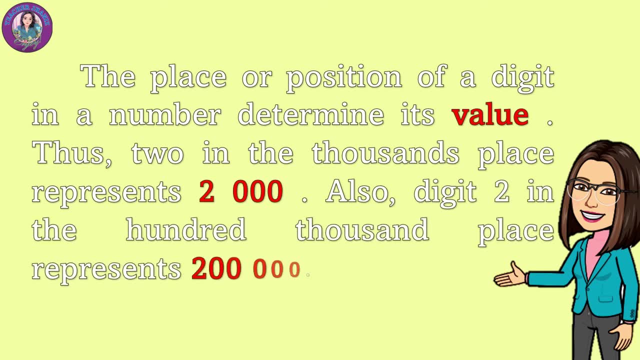 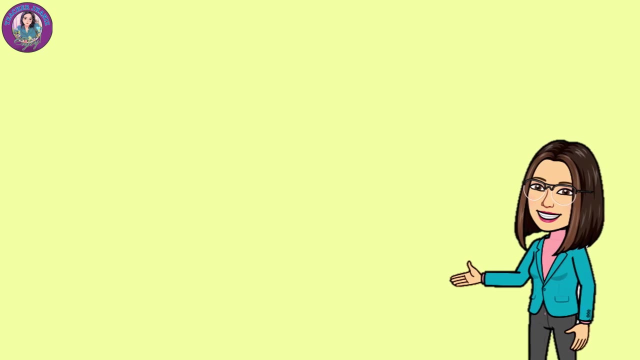 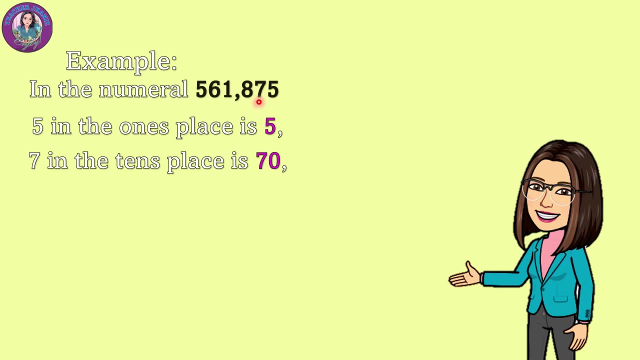 determine its value. thus, 2 in the thousands place represents 2000. also, digit in the hundred thousands place represents 200,000. example, in the numeral 561,875 the value of 5 in the ones place is 5. the value of 7 in the tens place is 70.